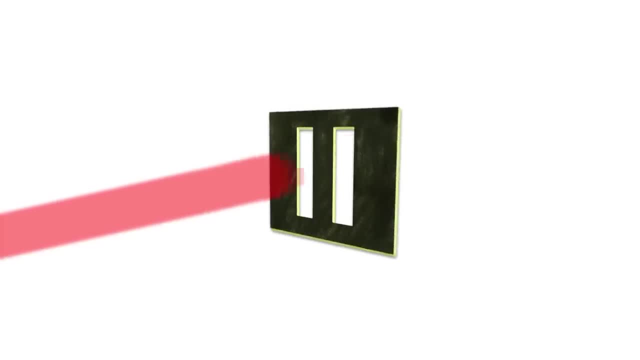 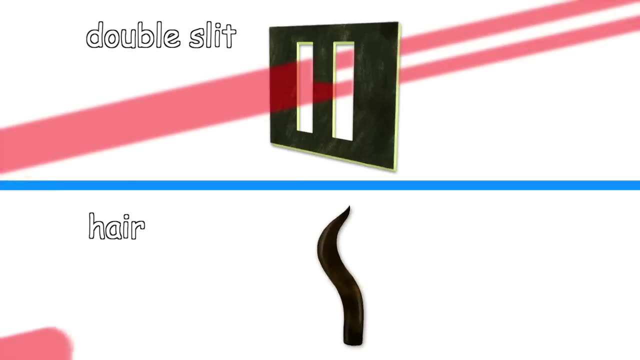 The normal way to do the experiment is to shine a light on two very narrow slits. Then the light that goes through goes through the left or to the right. This variation is pretty much the same. The light goes through one way and the light that goes through the other way. This variation is pretty much the same. The light goes through one way. 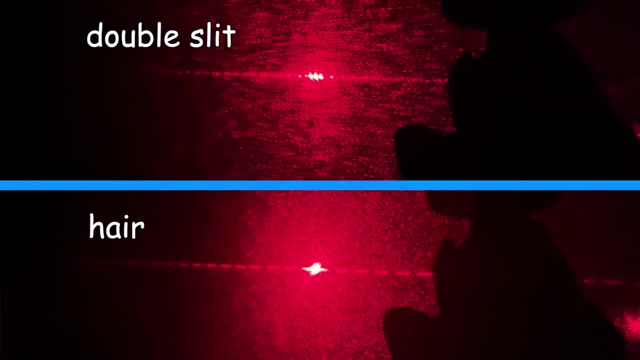 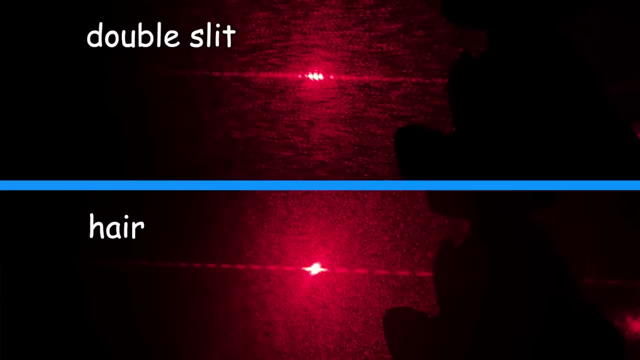 or the other. But besides being easier to do this way, the other advantage is the pattern you get. You can see that they both have the same sort of flavour, but they're different. For example, the dashes of light for the hair version are all evenly spaced. 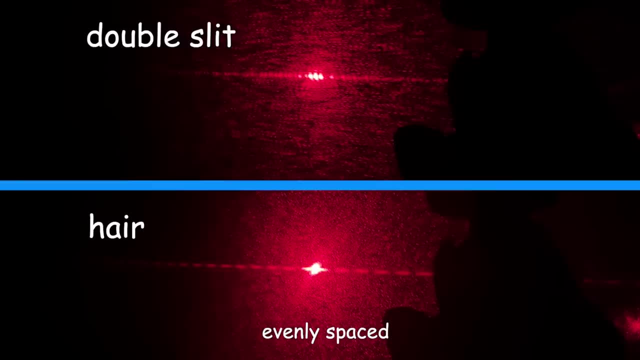 and get lighter as we go, But the dots of the double slit are much more patchy. That's because of something called single slit interference, which is basically a distraction in this scenario. So, yeah, I kind of prefer the hair version Plus, check this out, I'm using this. 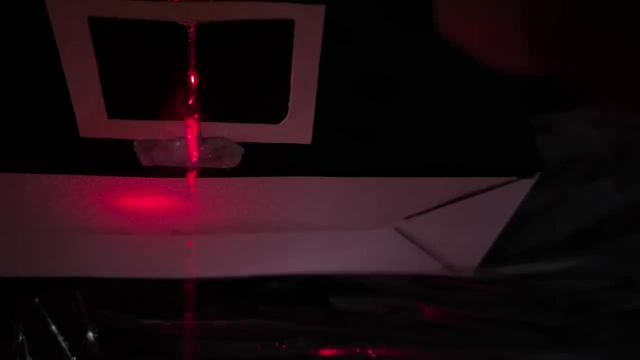 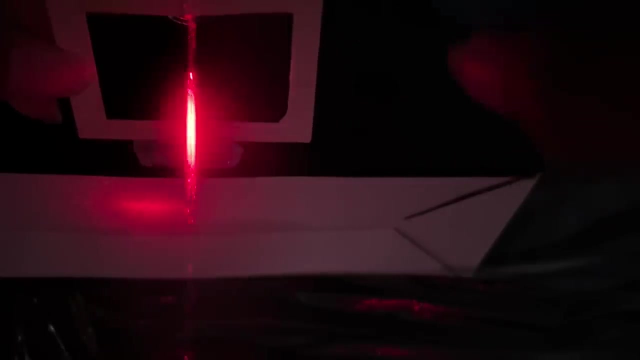 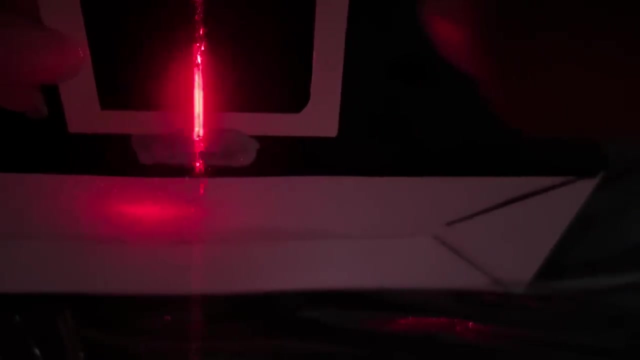 smoke-in-a-can stuff to see the actual beam. but look really closely at the beam and you can actually see where the hair splits the light into two. How crazy is that? And looking at this, I think it's really hard to understand why you get the crazy double slit pattern. 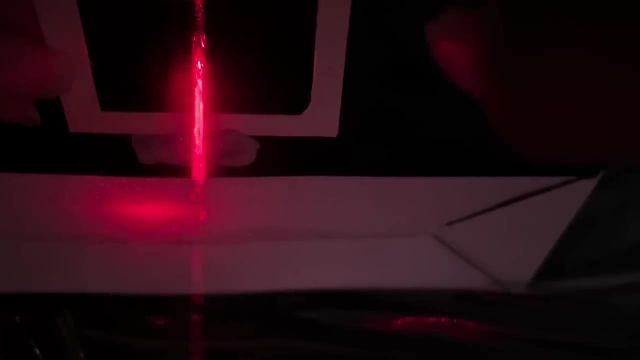 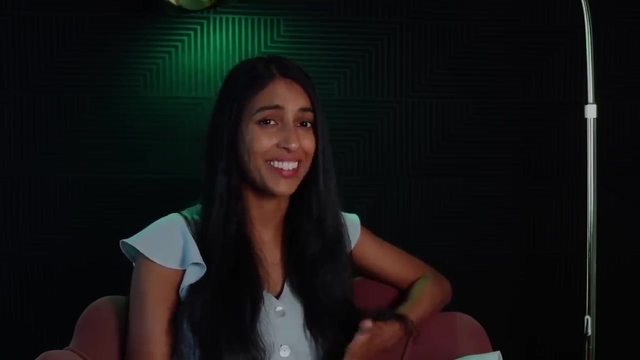 when it seems like obviously you should just get a dot with a line through it. So I've done my PhD in quantum stuff and I thought I understood the theory of this experiment really well, And so my plan was just to explain it to you in a cute 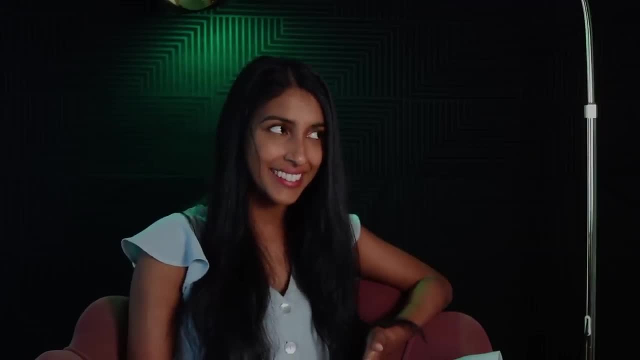 little video about how to do the experiment at home. Instead, I got sucked into an odyssey for the last few months where I did all kinds of variations on the experiment and I ended up like questioning pretty much everything I thought I knew about light. It turns out this experiment 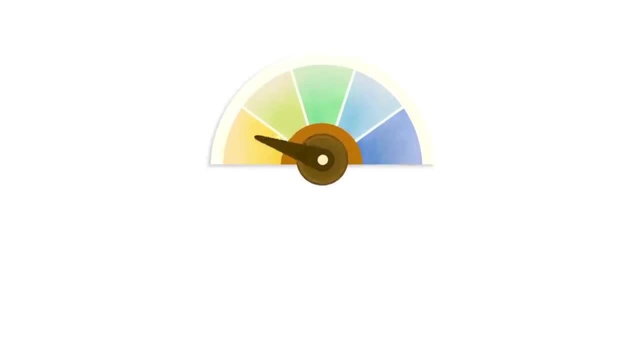 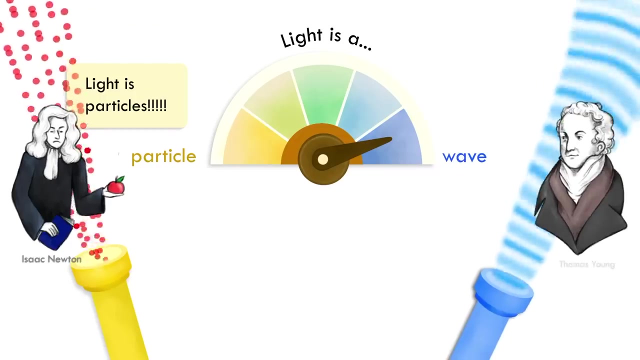 is just way more interesting than I thought. There's always been this debate in physics about whether light is made out of a stream of particles or light is some sort of excitation like a wave. The double slit experiment was meant to definitively prove that light is a wave. 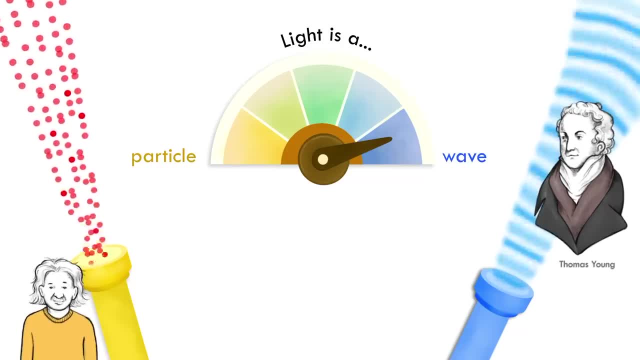 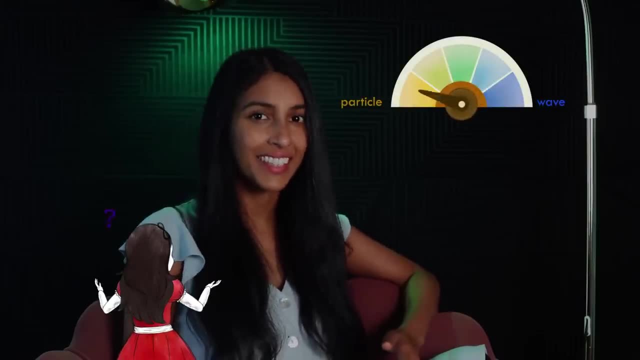 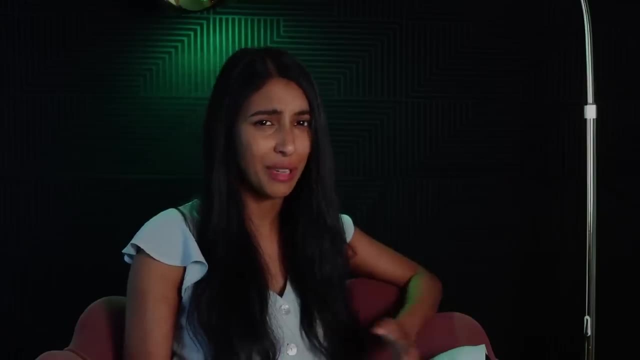 except later. experiments seem to show that light has particle-like properties as well. I used to hate this whole wave-particle thing because light is clearly neither. A great analogy I heard for it is that light is like a platypus. it doesn't make sense to say that it's both a duck and a beaver at the same time. 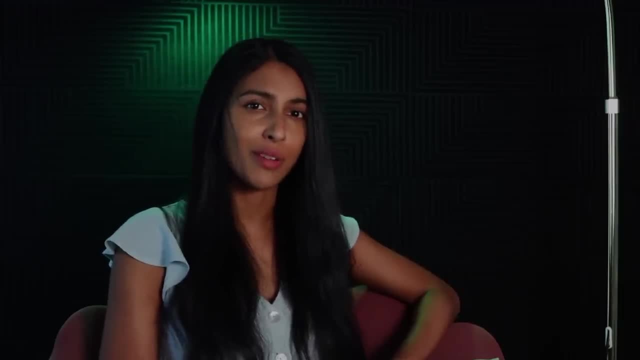 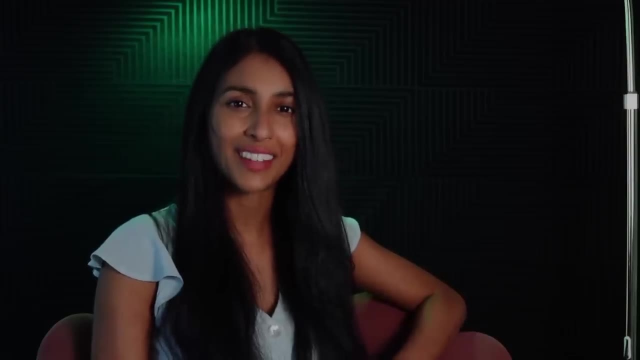 because it is its own thing. But actually doing this experiment finally made me see the value in having good analogies to help you think about light and in particular, it really sold me on thinking about light in terms of waves. It also made me see how misleading the particle analogy 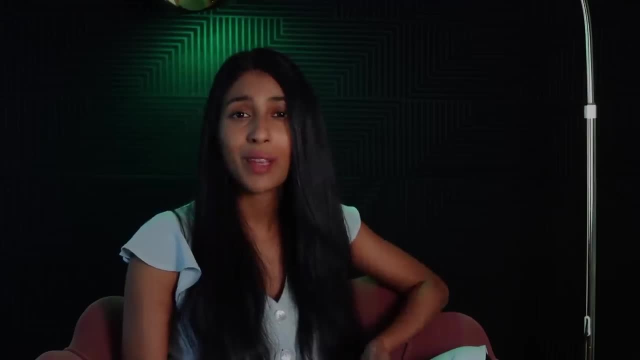 can be if you're not super careful about it. I think many of us imagine photons, which are what physicists now call particles of light, in a similar way to how Newton thought of light particles. But the double slit experiment shows why Newton's particle view is definitely wrong. 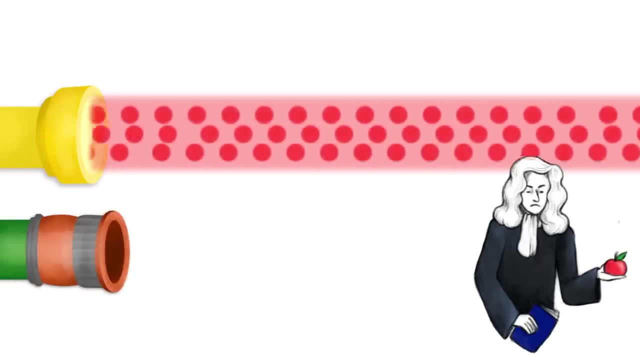 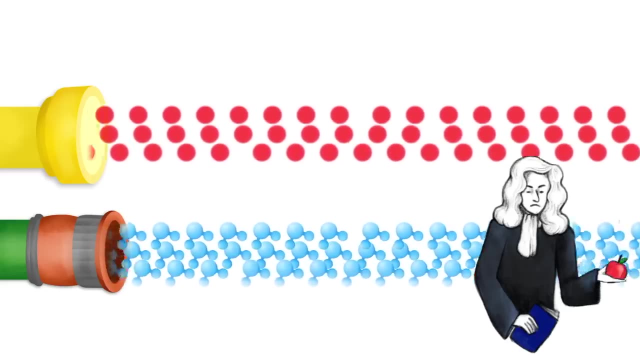 Newton imagined light in the same way we now think of water. Inside, it's just made of a stream of light particles, in the same way that water is made out of water particles. I'm going to call these particles that Newton thought light was made out of. 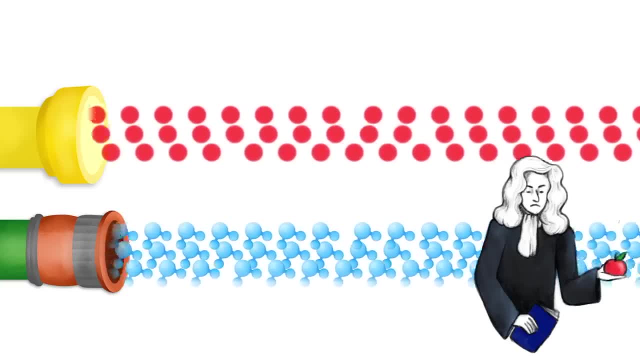 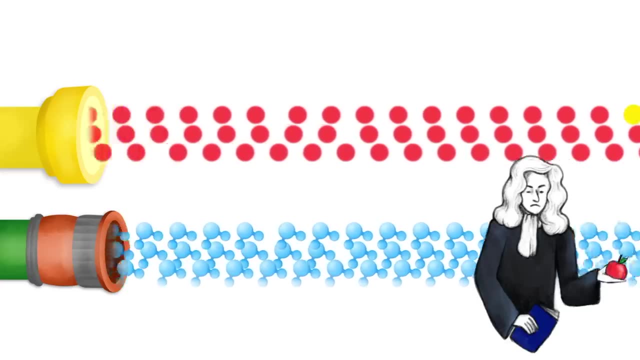 localized particles because at every point in time they're just in one spot in space. They're not in multiple places or very spread out or anything like that. If you turn down the laser, enough Newton would have expected that light comes out in these. 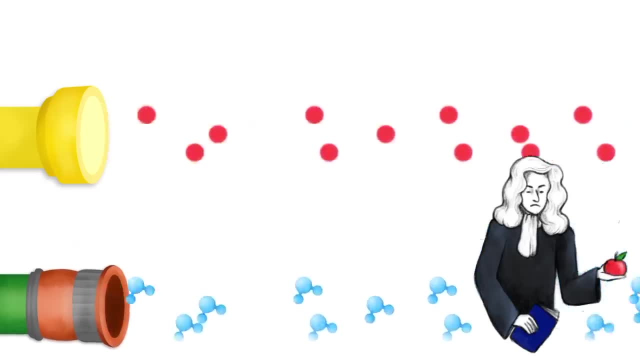 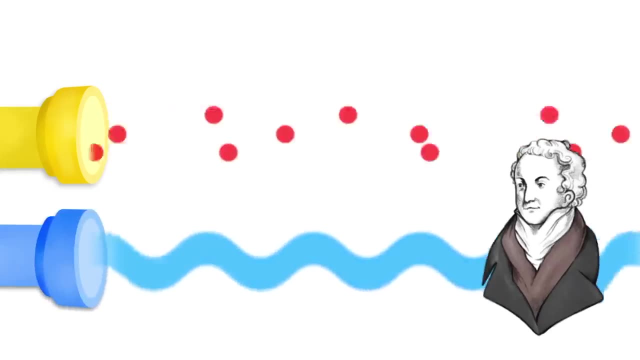 individual particles. Instead, people like Thomas Young imagine light coming out as some sort of wave. In this case, no matter how much you turn down the laser, the light would still be a wave. it would just be less and less wavy. The light travels forward, not in lines. 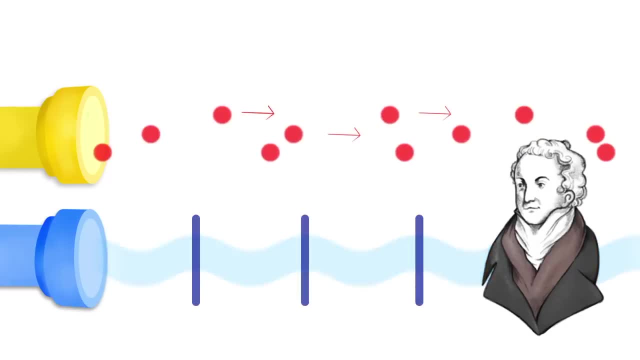 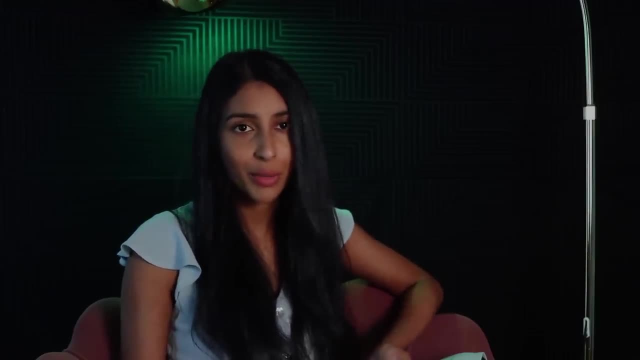 but as peaks of a wave progressing forward. In the case of just turning on a flashlight, both Newton's picture and Thomas Young's wave picture make exactly the same predictions, But Newton's view just feels bright, Like you have these particles just traveling in straight lines. 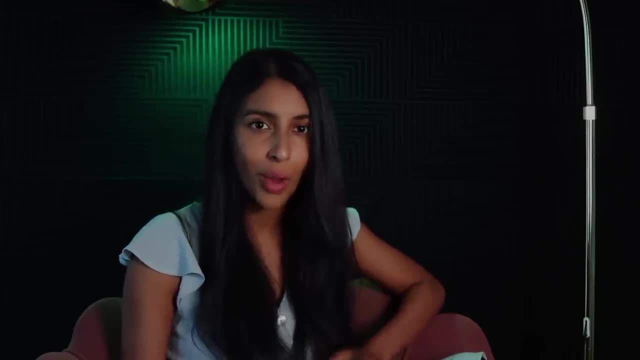 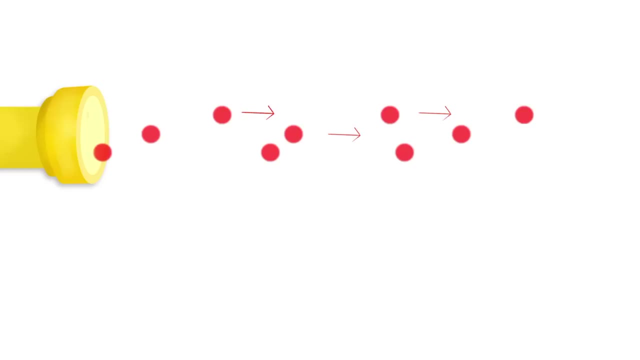 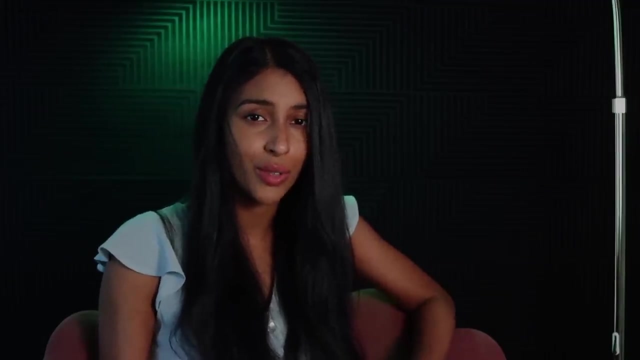 which is so much simpler than this strange abstract wave thing, Which is why it's so tempting to think of light this way. In fact, I've seen pictures just like this one to illustrate photons exiting a light source in many reputable textbooks, And I get why. that's kind of how I imagine photons too. 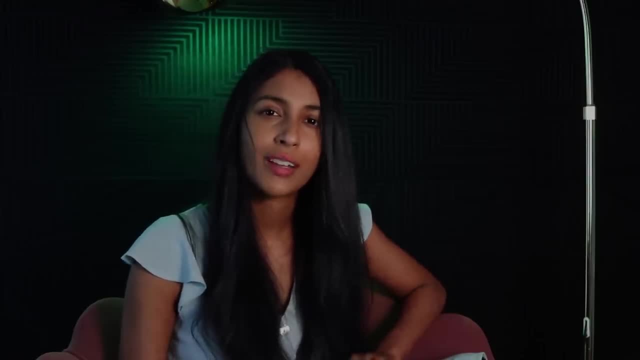 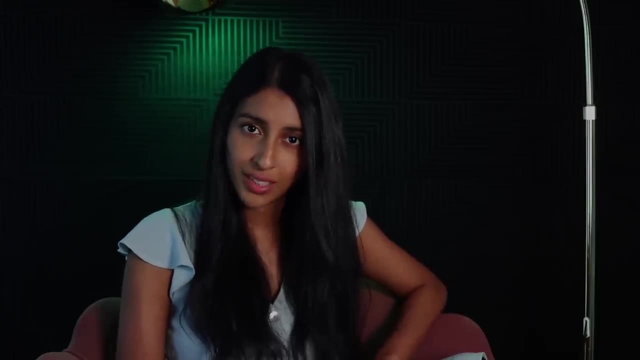 So how did Thomas Young go about disproving it? He needed to find an experiment that could only be explained with waves and not with Newton's particles. Well, one unique thing that waves do is that they bend and spread out. You may have seen this before. 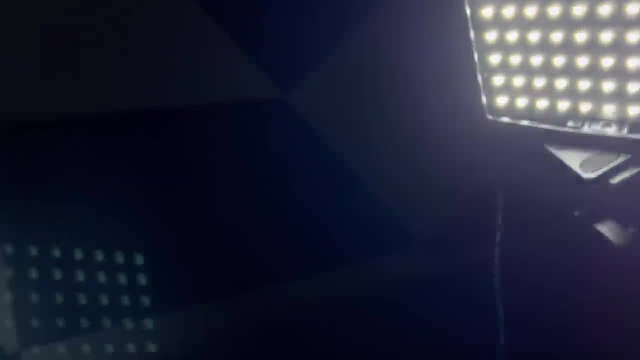 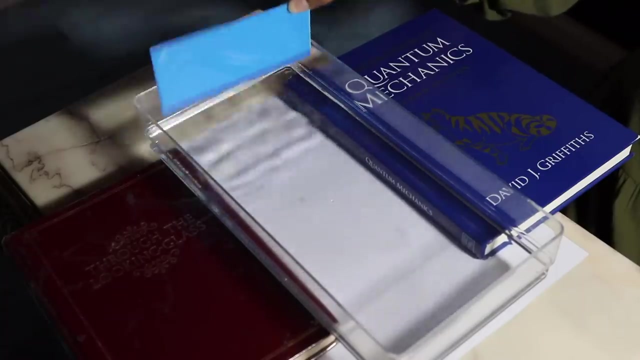 but for me at least, it was kind of surprising. Let me show you with this high-tech ripple tank I made here. You can see that when I bob this plastic in the water it makes fairly straight waves. But what do you expect will happen when I put this obstruction in the way? 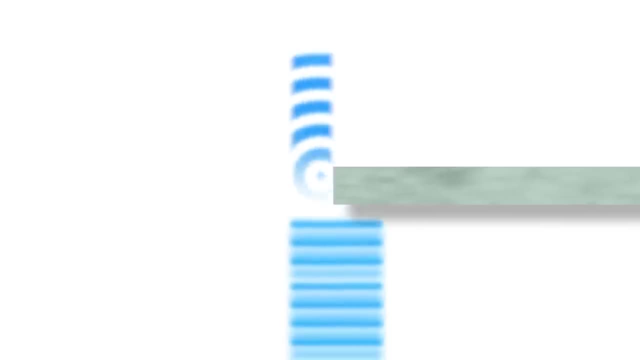 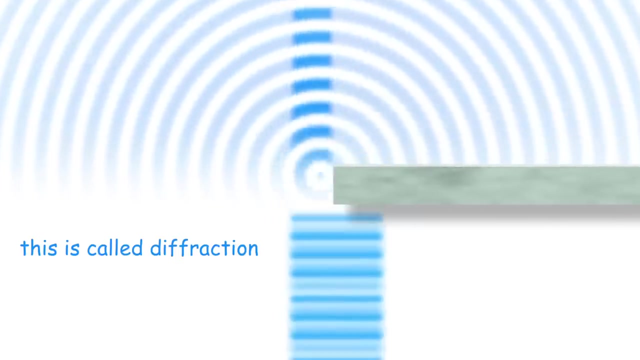 I would have guessed that the bit of the wave that makes it pass just goes straight ahead, and that's what the majority of the wave does do, but the rest of it bends and spreads out. You can see that in action here, But why does it happen? 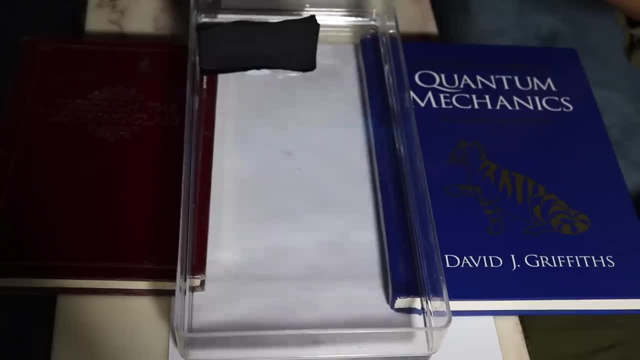 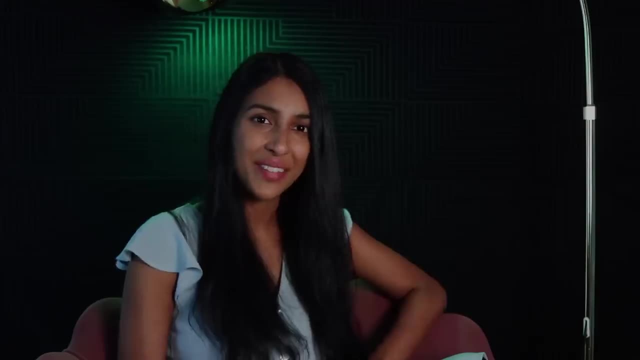 I don't really know. I would love to understand it better and make a video about it, but until then, you can see that this is something waves actually do. They spread out when they meet an obstacle. That definitely feels a lot different from how I'd expect particles to behave. 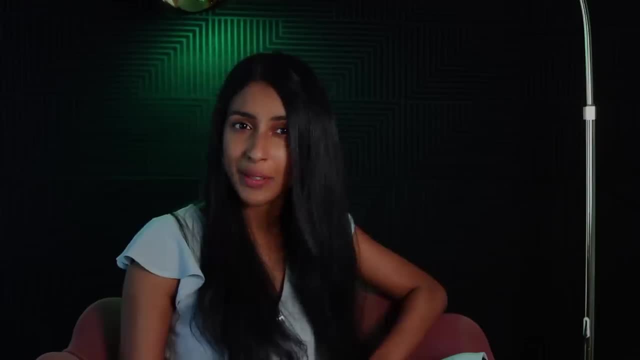 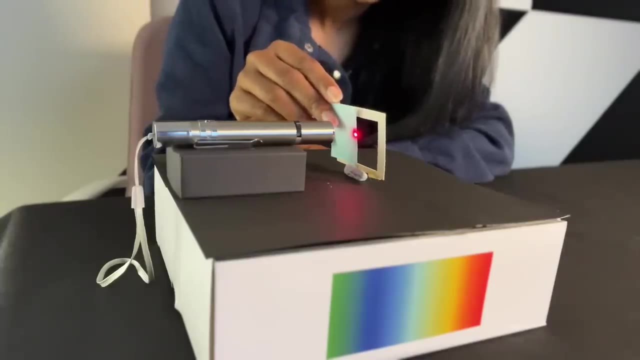 So why don't we do a similar experiment with light and see what happens? Will light bend and spread out, or will it go straight? I'm going to use a piece of paper as the obstruction to find out. And there you go: The laser light does actually spread out. 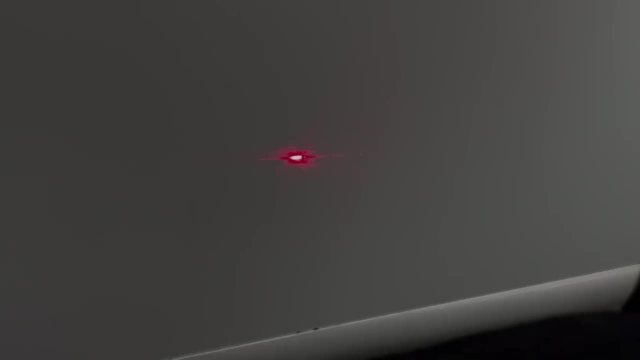 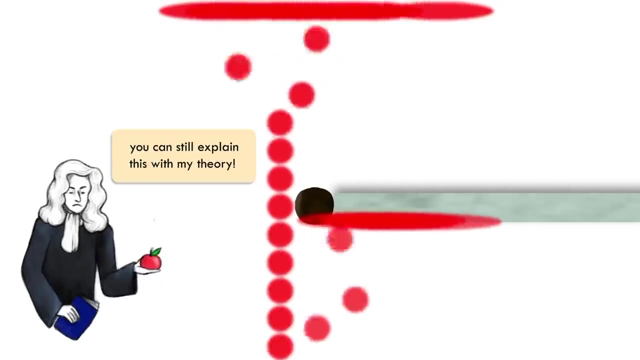 I'm going to use a piece of paper as the obstruction to find out. Case closed. Light is a wave right. Well, maybe we should give Newton a chance to rebut this. I guess he could try and explain this with particles. Perhaps the particles are colliding into the paper and then ricocheting. 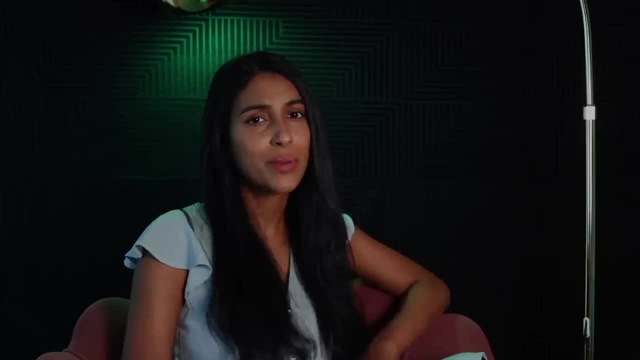 and that's why they spread out like this. Okay, fine, Maybe you can explain that, But there is another wave phenomenon that particles definitely can't mimic, and that's cancelling out. One way to think of the last experiment is that it's like we took the hair experiment and then 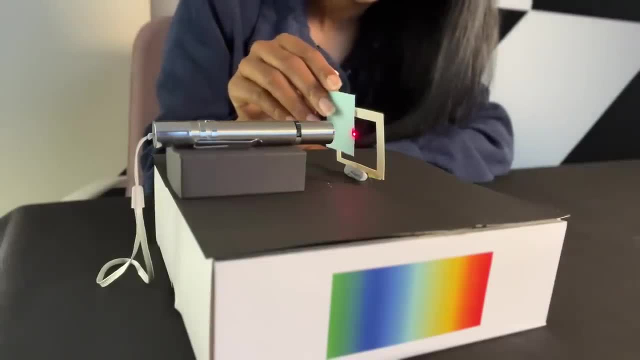 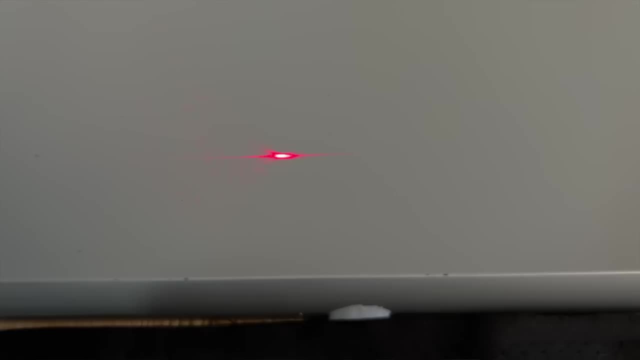 just blocked one path, We found that at least some of the light ends up in all of these places, including in this spot. If we had blocked the right path instead, we'd have gotten a very similar result And again notice that at least some of the light falls on this spot. 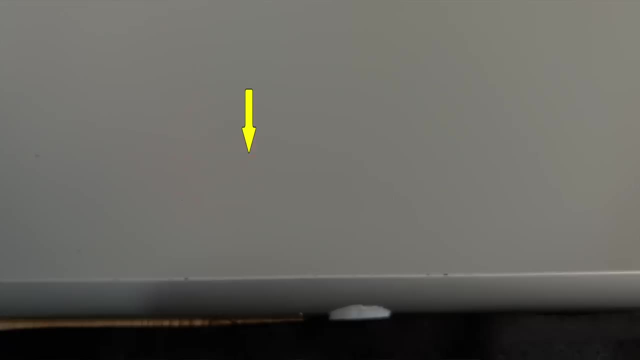 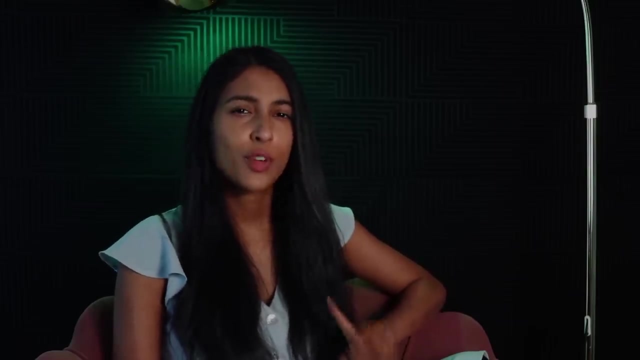 Now let's open both paths simultaneously and the light just disappears from this spot. There is no way for Newton to explain this. Think about it. If you believe in the kind of particles that Newton did, then when just the left path is open, some of your particles will reach that spot. 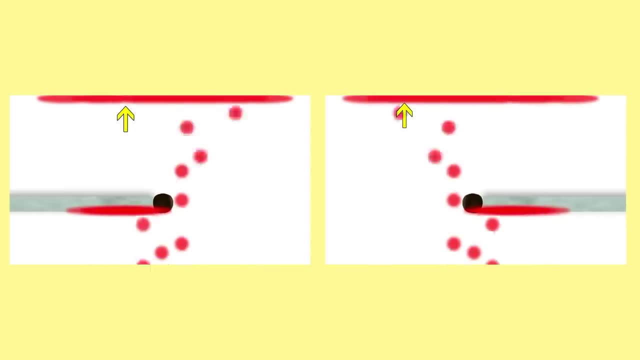 And when the right path is open, some of your particles will reach that spot. But when both of them are open, it's like the particles from the right side and the particles from the left side just happen to cancel each other out in this spot. 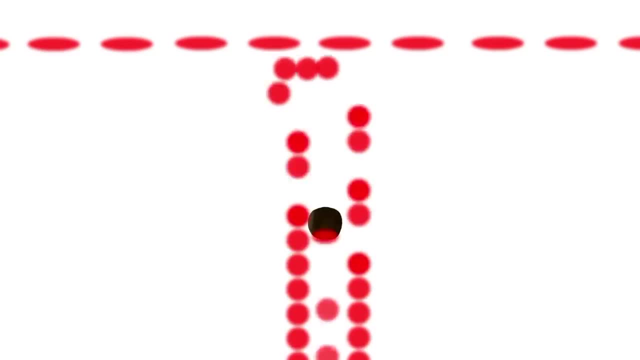 Which just doesn't make sense. But why not? Why can't you just have the particles cancel? Well, because in this spot they need to cancel, But just a little bit over. the particles coming from the left and from the right should happily coincide. It's like they sometimes choose to. 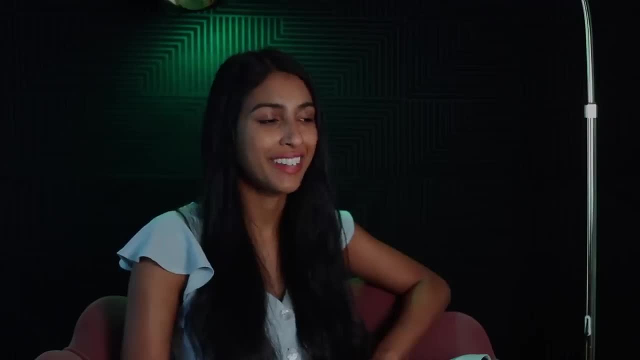 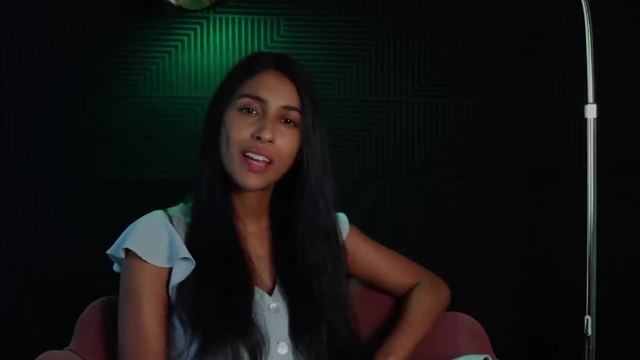 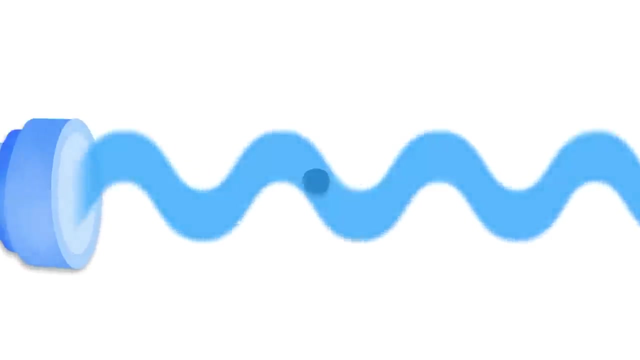 cancel, and sometimes they choose not to. So I'm sorry, Newton, but particles like yours really aren't good enough to explain how you could ever get cancelling. But then how do waves manage to explain the double slit experiment? Let's imagine a wave is coming out of the laser. On the right side, the wave encounters the hair. 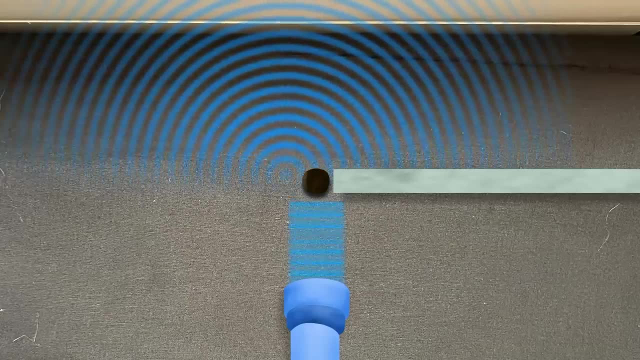 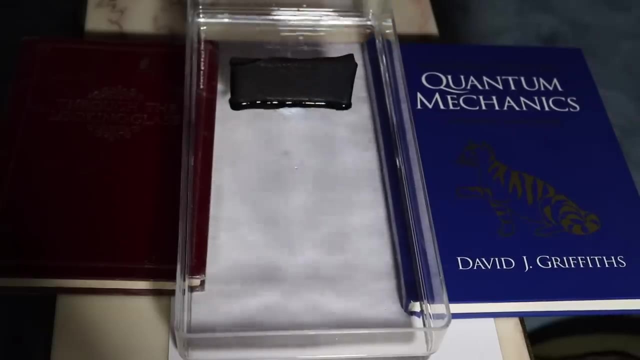 and, because it's an obstacle, it bends and it spreads out, like we discussed before. On the other side, the exact same thing happens Back in our wave pool. the black obstruction in the middle now represents the hair And, as you can see, the waves on either side do spread out and they overlap. 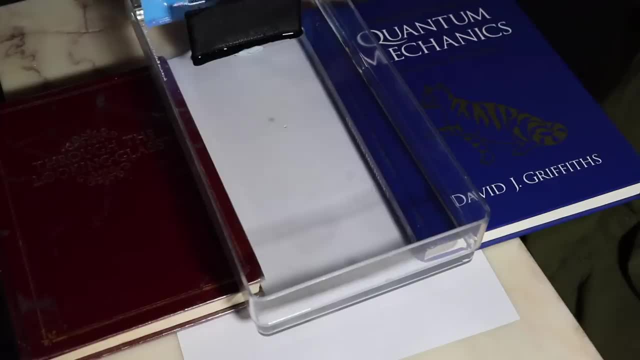 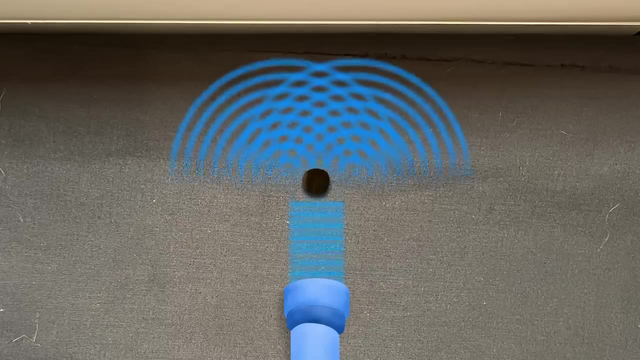 But something very surprising is happening in that overlap and you can't really make it out in this precision setup, but it's going to be a lot more clear in the animation. Where are all these lines coming from To understand what's going on? 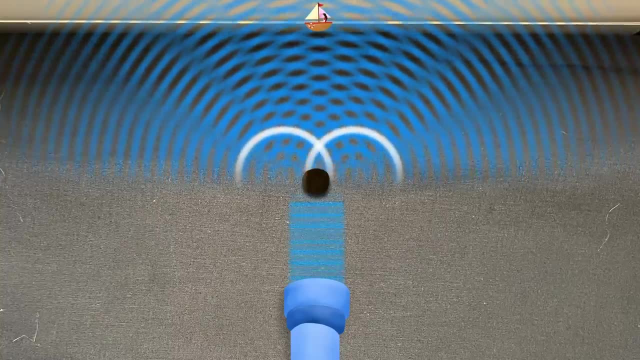 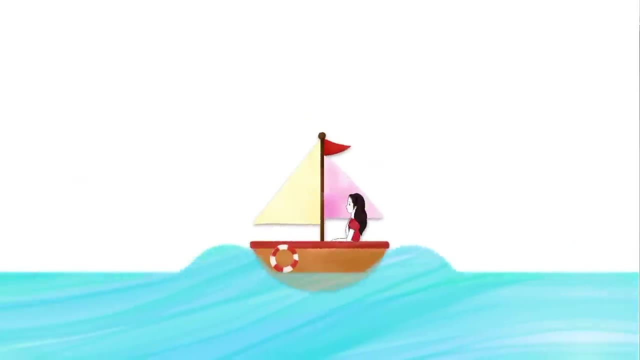 imagine you're on a boat in this spot. Then the wave coming from the left will have its peak, reach you at exactly the same time as the wave coming from the right. Together they tend to push you up even higher. The troughs also meet you at the same time, so this spot is just really choppy. 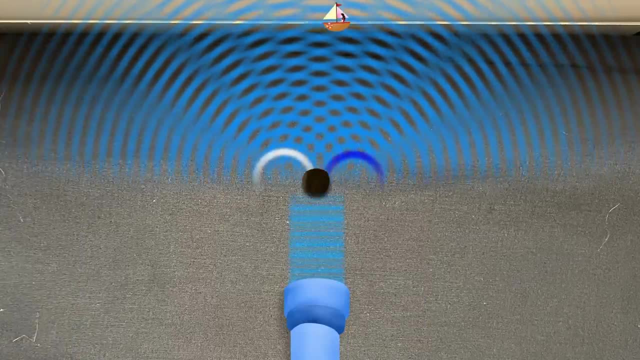 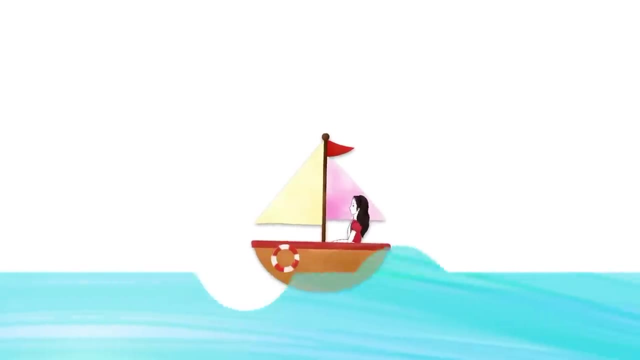 But if we instead move our boat to here, then the peak of the right wave hits exactly when the trough of the left wave hits you. The peak tries to move you upward, while the trough tries to pull you down, And so in the end they cancel out and the boat doesn't. 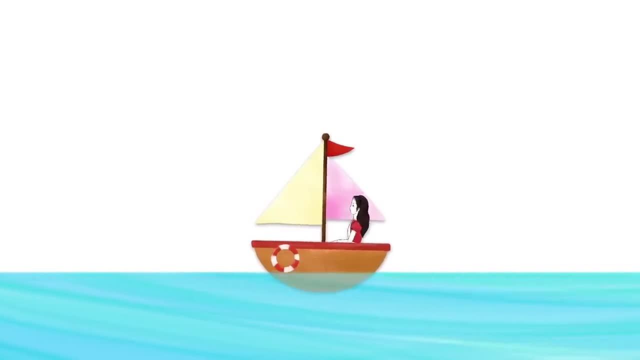 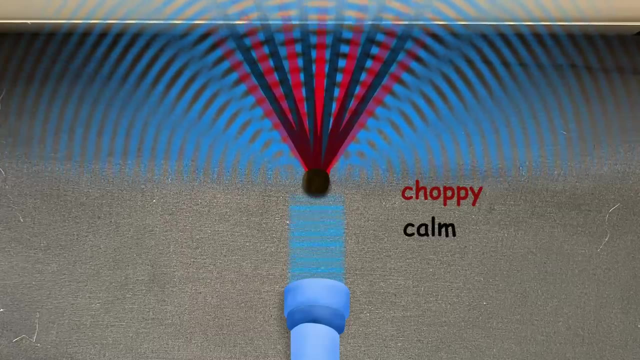 really move up or down, So this spot is surprisingly calm. There are these choppy and calm spots all over, and if you map them out, then you get these lines. What's this got to do with the double slit experiment? Well, look at the waves across. 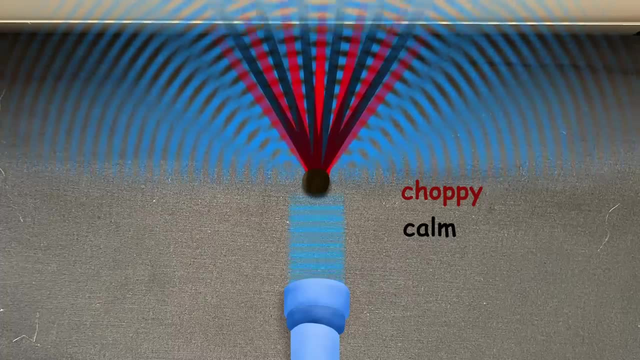 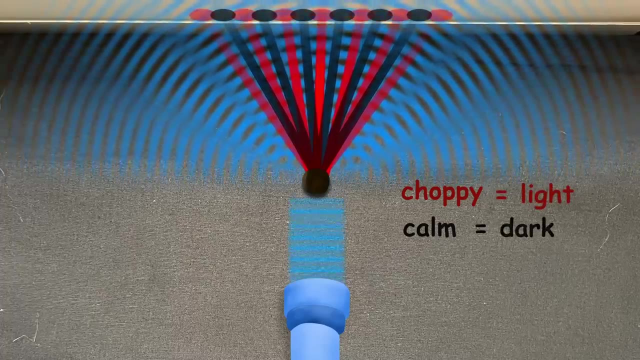 the wall You have these alternating parts of choppiness and calmness. That lines up suspiciously well with the pattern of the double slit, where you have alternating spots of light and dark. Thomas Young's hypothesis was: when there's this waving, 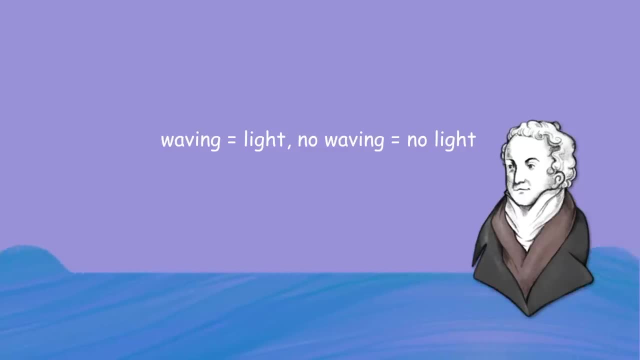 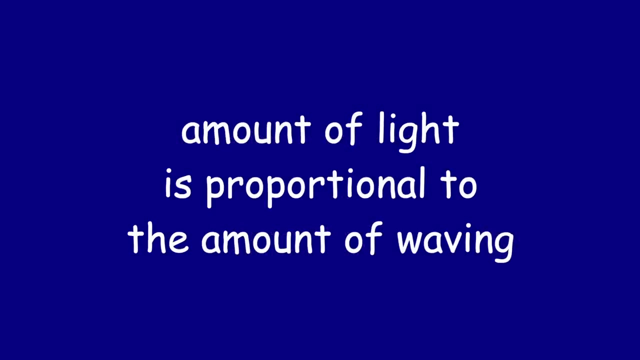 there's light And when the waves cancel out and so there's no waving, there is no light. In other words, the amount of light produced in a spot is proportional to the amount of waving. You know, I've given this explanation to students for years, but I've never taken the whole wave. 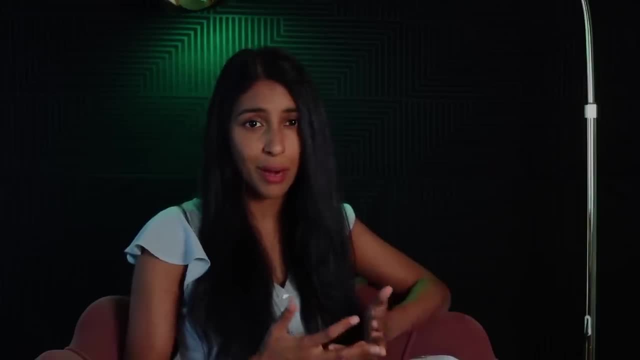 picture very seriously, Like: yes, I knew that to make the right prediction for the double slit you would have to use waves in your calculation. But I thought they were just that, you know, like just calculation tools. I thought they were just that, you know, like just calculation tools. I didn't think that they were. 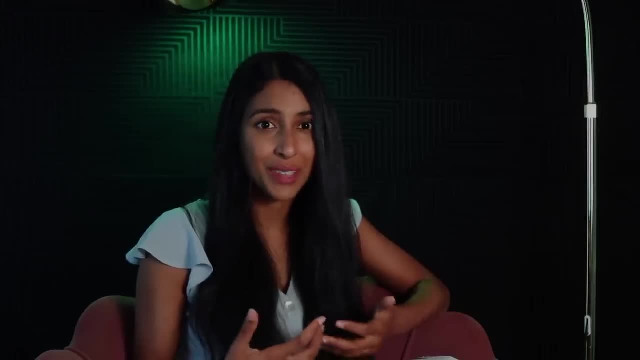 just that, you know, like just calculation tools. I didn't think that they were just that. I mean, like, literally, in quantum mechanics the waves are complex valued. So instead in my head, you know, I thought of the light as a particle when it exited the laser. 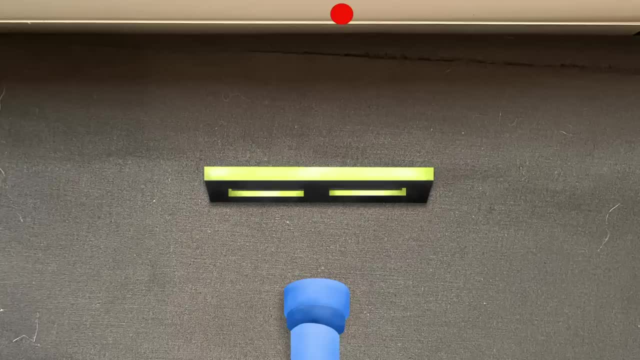 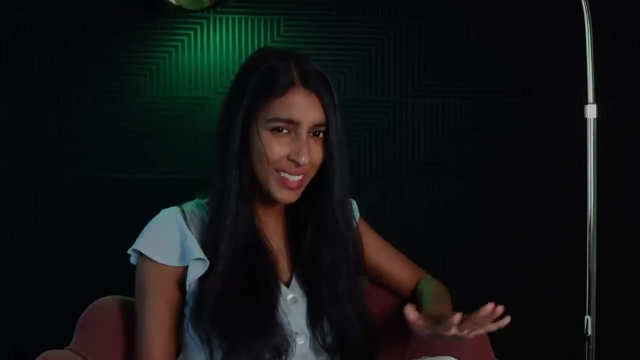 and then a particle again when it got measured at the wall. But in between it just seemed like there's nothing you could really say about the light besides a bunch of equations. But this next experiment is what changed my mind and made me finally feel that the waves 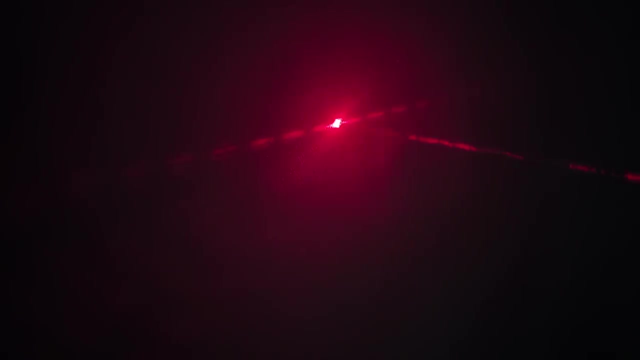 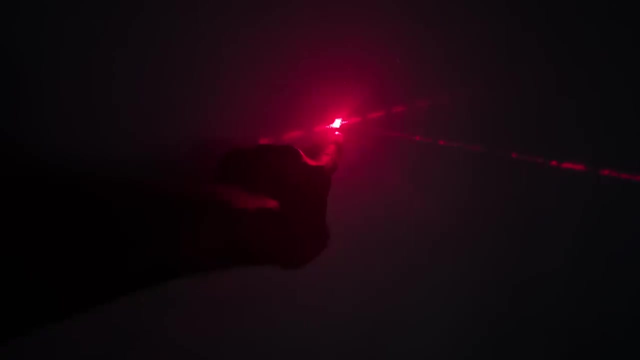 are actually real. So I've been playing with this for a while and I haven't been able to get this thought out of my mind. There's a beam here that leads to this middle dot. That's clearly where the light for that dot is coming from right. But what about all these? 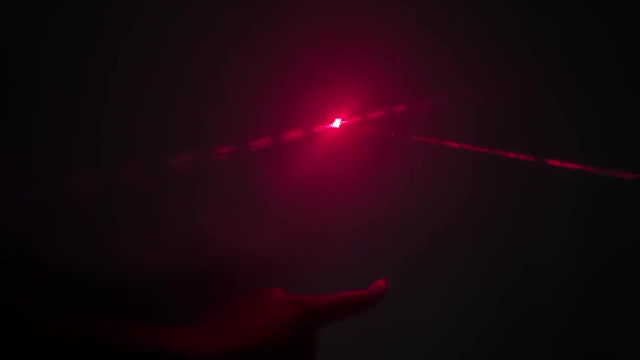 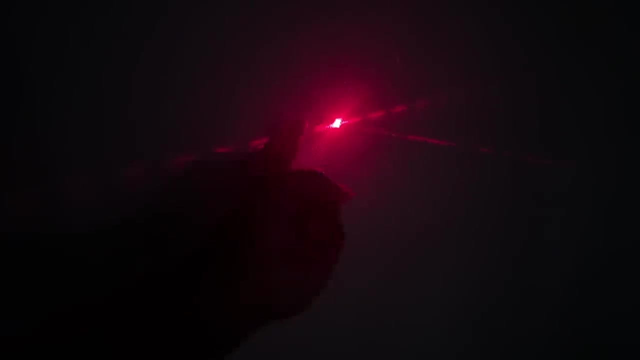 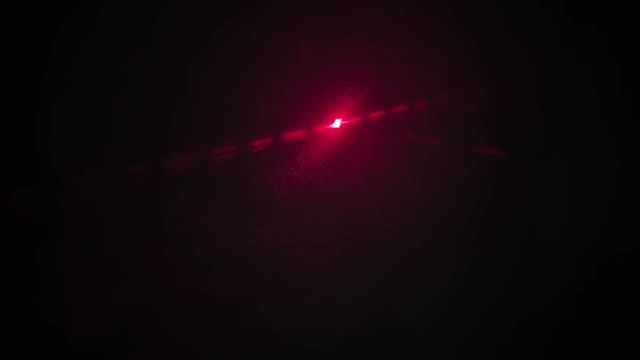 other dots, Like: surely that light is coming from somewhere as well, And it feels like you can almost trace back exactly where that light's from. For this one, if I follow it, I can go all the way back, And same for these as well. 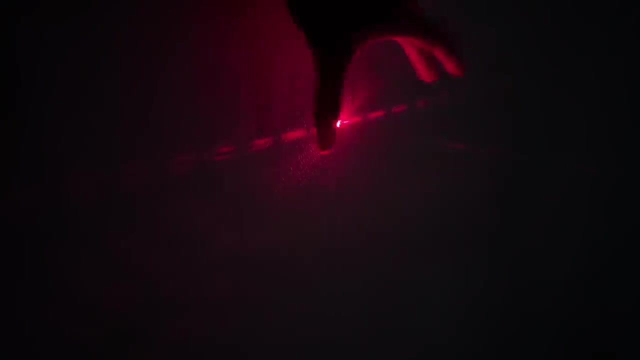 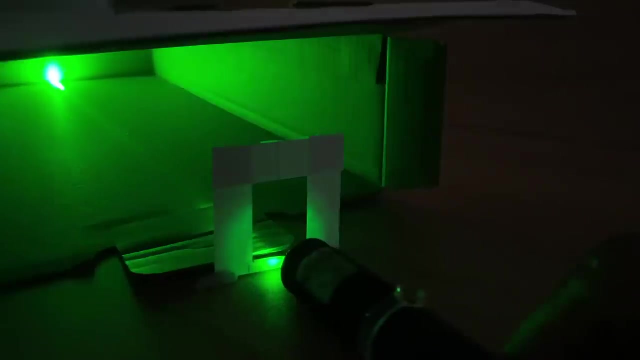 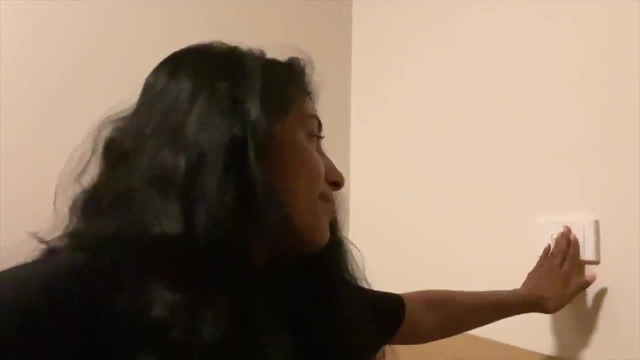 It feels like there should be beams kind of coming out here. I got obsessed with this idea that you should be able to see these beams of light if you just use the right method. I tried everything, Like doing the experiment of midnight for maximum contrast and then filling a box with smoke. 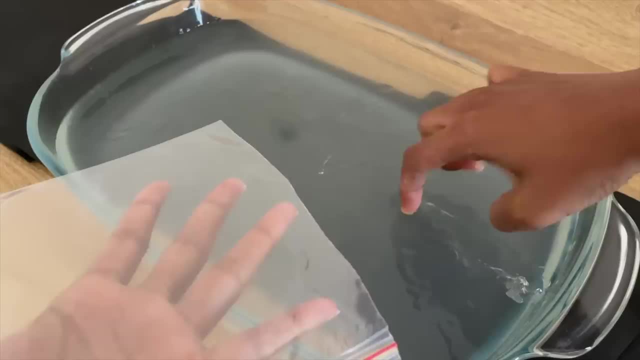 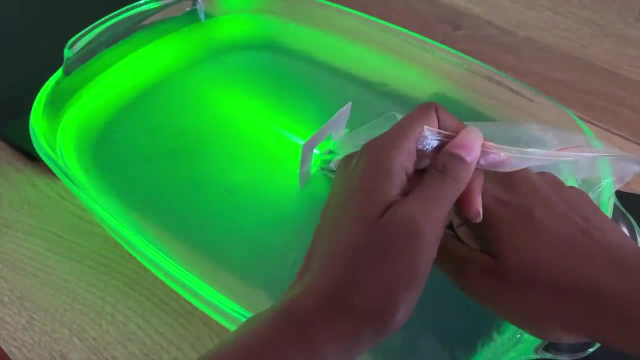 Then I tried the experiment at night for maximum contrast, and then filling a box with smoke, tried filling a tub with water vapor, I even tried submerging my laser into agar. Nothing. In the end I caved and I bought a smoke machine from a DJ shop And I also decided to use the 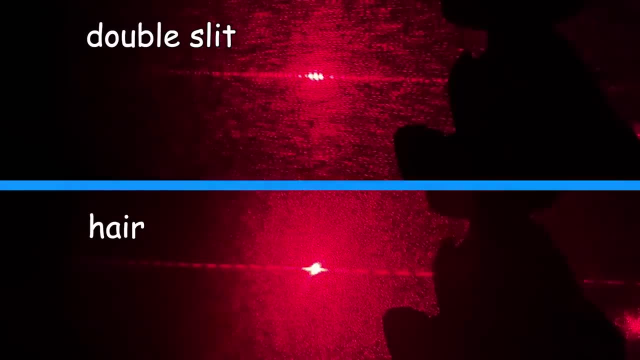 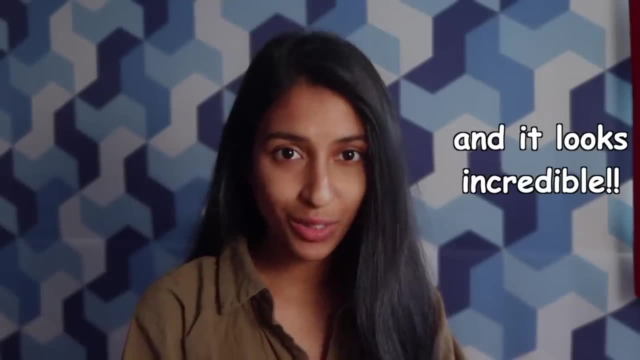 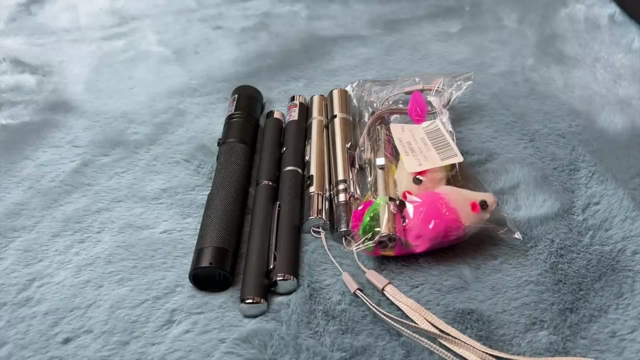 proper double slit so that the little bands are more intense. And it worked. I would love if you actually tried this experiment yourself, because it's so easy to do. But I need to warn you about something: Laser pointers are way less safe than you probably think. I bought a bunch of lasers from 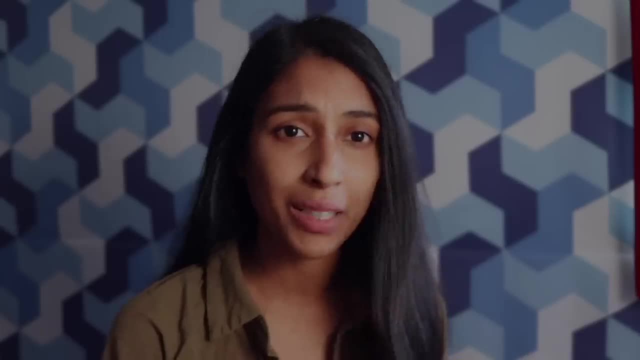 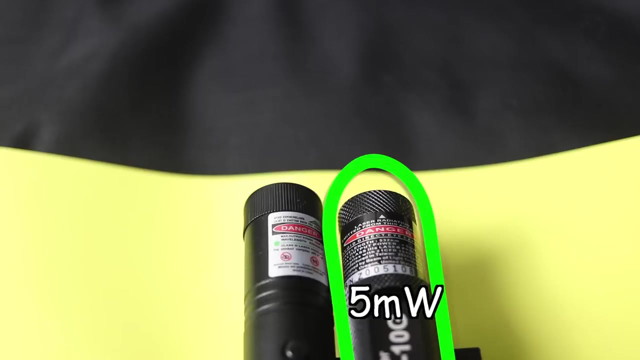 Amazon that all claim to be under five milliwatts. Anything over that limit can permanently burn a hole in your retina. So let's compare these cheap lasers with a proper five milliwatt laser to see if they're safe. As you can see, this green one is definitely not okay In general, green lasers. 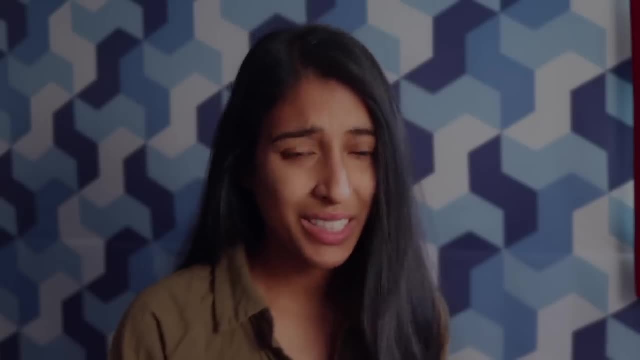 are something I really don't recommend you buy from Amazon. Red laser pointers are better in my experience, especially little ones like this that are advertised as like keychains or cat toys, But I don't recommend you buy them. I don't recommend you buy them. I don't recommend you. 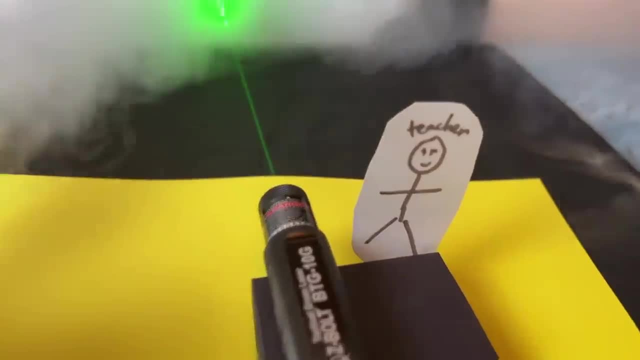 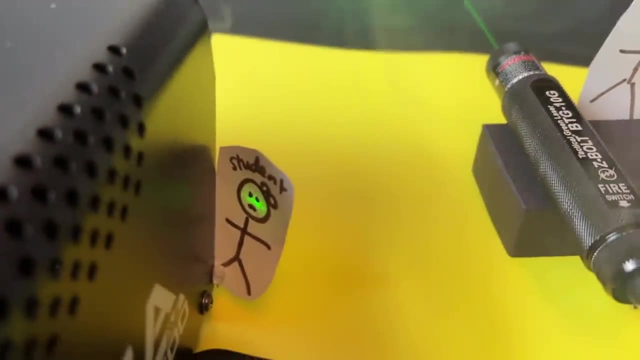 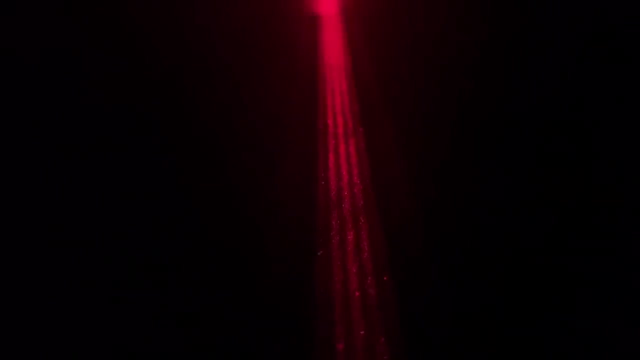 buy them. But yeah, if you're going to be using a laser for presenting or experiments or playing with your cat, just make sure it isn't one that's going to burn someone's eyes out. Anyway, it was worth buying the smoke machine. This experiment looks just magical in real life And all I've 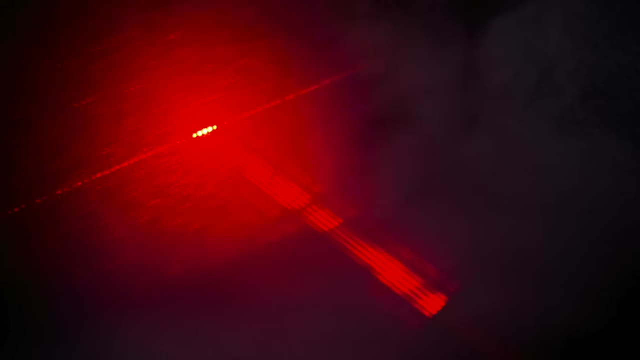 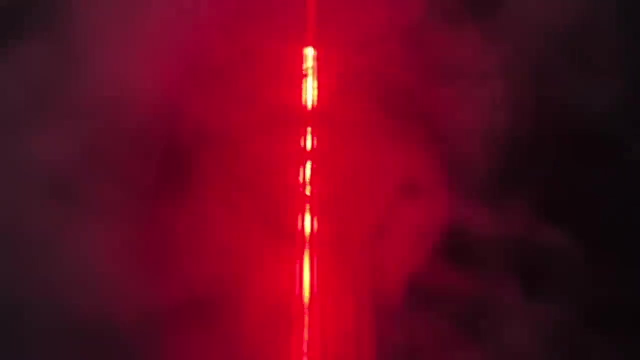 done to capture it is: use my phone, Nothing fancy. I set the double slit up a few meters away and locked all the lights and turned on the smoke machine And all of these beams suddenly became visible. Here you can see that there are beams of light going to all of the dots of the 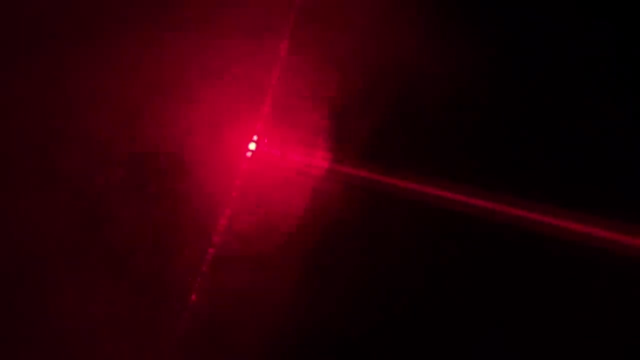 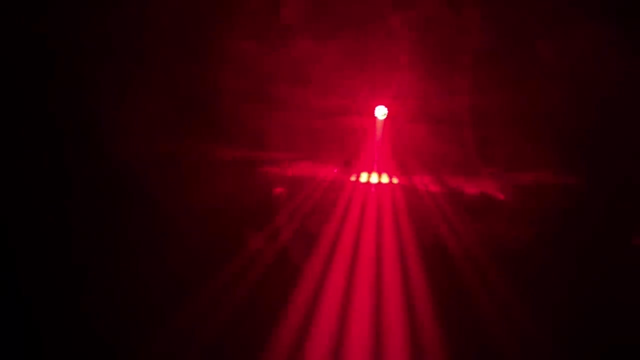 double slit pattern. But to see it even more clearly, let's turn around and look toward the laser. And now so many beams become visible. The double slit doesn't split the light up into two beams. It splits the light into many, many beams. So why was this experiment such a revelation for? 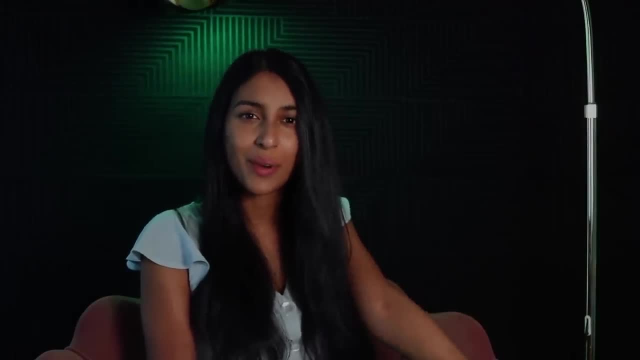 me. Well, it felt like I was actually seeing the light, but I didn't know what it was. I was just trying to be a wave. for a first time, Let me show you what I mean with this laser. Here you can see. 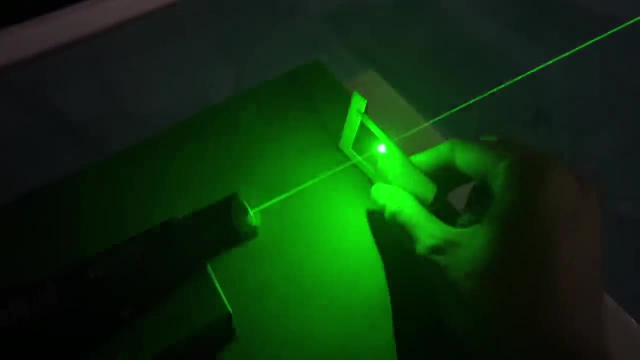 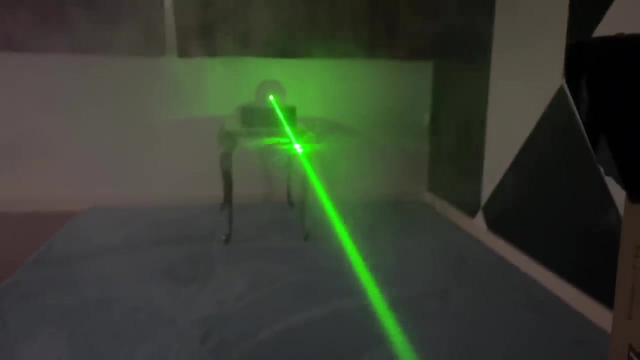 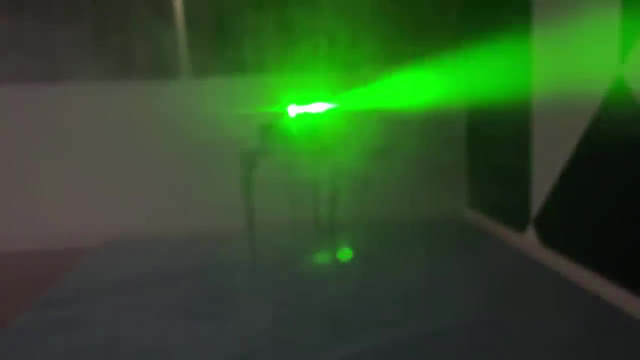 the narrow beam of the laser, but if I put this paper in the way, a wave should spread out. And yeah, that's exactly what the laser does. But to see it more clearly, let's add some smoke. This looks almost unreal. The laser beam is spread out, but only in this one plane.